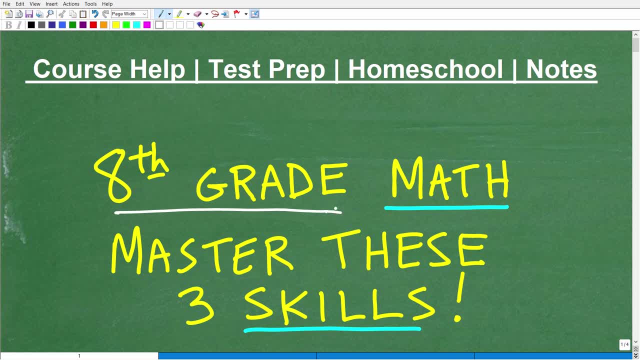 Maybe you didn't finish the eighth grade, Maybe you got a GED later down in life. My father, actually, I think he only went through like the seventh grade, And then he joined the army when he was 17 years old, And by the time he was 18, actually, while he was 17, he was actually in the Korean War, So that's how they used to do it way back in those days. He didn't really have, you know, a huge education requirement to go into the military, So, but here's the thing, though you know, even like my dad, he got his GED. 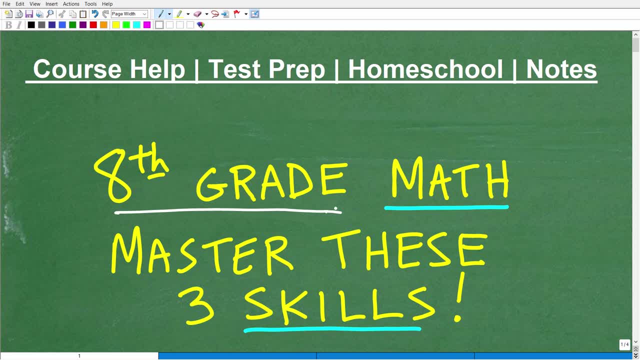 And then you know he did fine later down in life. So what I'm trying to get, the point I'm trying to make, is, if you didn't finish your formal education, that has nothing to do with your current potential. I'm probably already telling you something you already know, And if you're like boy, I want to go back and, you know, relearn this stuff. Or you know, maybe you are in eighth grade, maybe you're a parent of an eighth grader. Listen, I'm here to tell you that the eighth grade is pretty important. All right, You know we're all focused on algebra and all that kind of stuff. 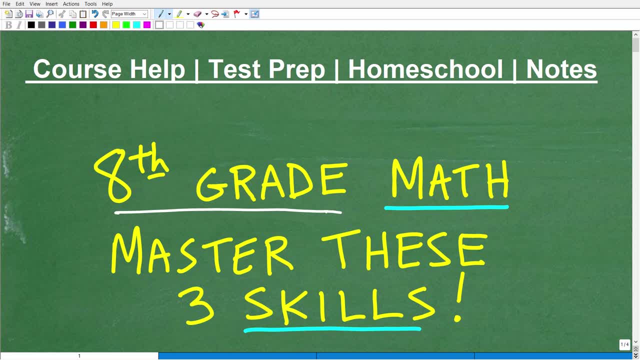 But if you don't have a GED, you're not going to get a GED. If you don't get these three skills right in the eighth grade, at the eighth grade level, the middle school level, you're going to have a tough time. But if you get these right, you're going to really set yourself up nicely for success. I want to talk about these three specific math skills in just one second, But first let me quickly introduce myself. My name is John. I'm the founder of Tablet Class Math. I'm also a middle and high school math teacher. I'm going to leave a link to my math help program in the description of this video. But if you're having a tough time in math or maybe you want to get a GED, you're going to have a GED. 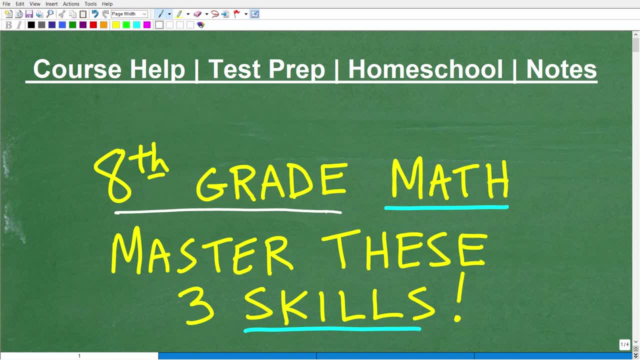 If you want to go back and relearn a lot of math. well, you know, the key is this One: you need to have the desire and work ethic. You know you've got to be willing to work hard and study hard to learn math. That's not going to change no matter what. But the second part of the formula for success for math is instruction. You need a teacher that you like and understand, And I believe I can be that teacher for you. I've been teaching math for decades and I do not teach like a textbook. I really focus in on explaining math and super clear and understandable math. 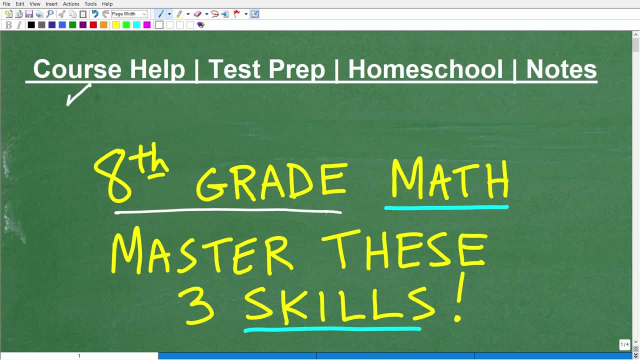 So if you're at the middle school, high school or college level in terms of mathematics, please check out my math help program. It will definitely help you out. Now, if you happen to be preparing for a test that has a math section on it- I am talking about things like the GED, SAT, ACT, GRE, GMAT, ASVAB, ACCUPLACE or CLEP exam, maybe a teacher certification exam- I can help you prepare and pass those exams. 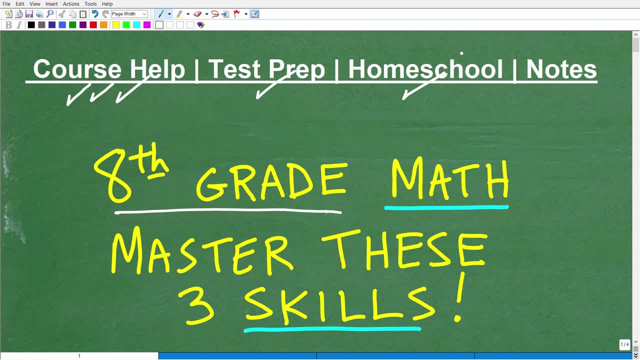 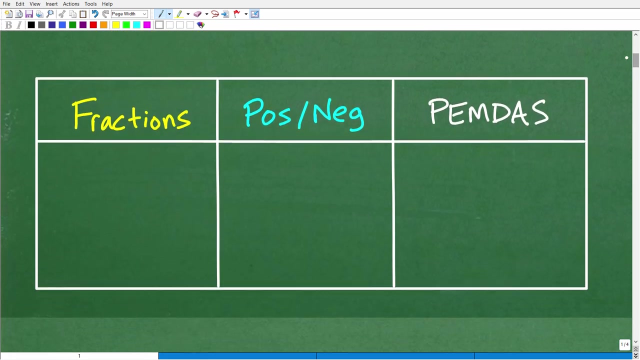 If you homeschool, we were just voted number one Our math course. we were voted number one for the middle and high school math category by a major homeschool publication, national publication. We're very proud of that achievement. And if you don't have any math notes, I'm going to leave links to my math notes in the description of this video. But if you happen to be a math student, okay, the secret to getting great grades is by taking great math notes. Okay. so let's get into these three specific skills, Very, very important, And let's go ahead and talk about them right now. Now, the first thing is: 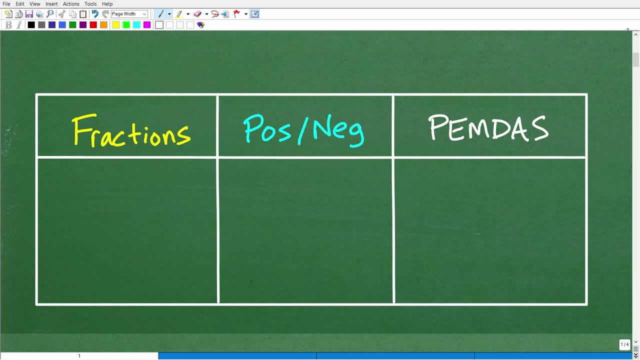 this: You're going to continue to practice these skills beyond the eighth grade And you probably learned a little bit about these skills prior to the eighth grade. But the eighth grade, okay. after you finish eighth grade math, for the most part most students are going to be going into pre-algebra And pre-algebra. it sounds like a course that you take prior to learning algebra, right? I mean, that kind of makes sense, right? It's like pre-algebra. So you got one more course. 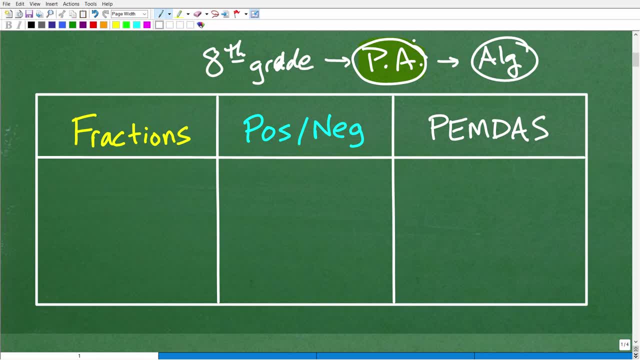 where you take algebra. Well, that's not really true. In pre-algebra you really are learning algebra. okay, It is your first real formal algebra course. It's just not as, let's say, as demanding of what you're going to be learning, like, let's say, in high school algebra. But you 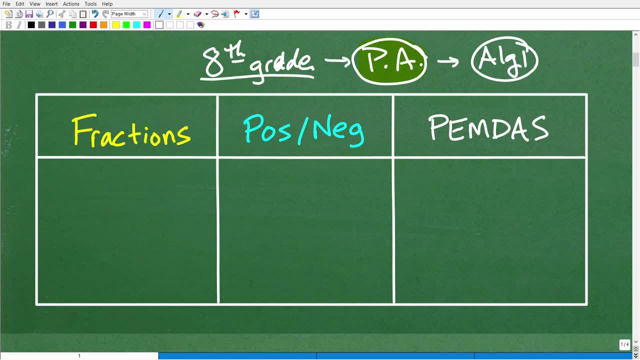 are learning algebra. So the eighth grade is kind of your last truly middle school level arithmetic related type of course. So let's take a look at these three skills, Super important. If you get these down, you're going to be very prepared to be successful in pre-algebra and any course. 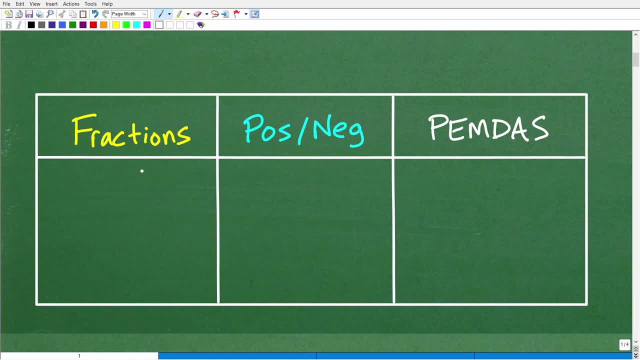 beyond that? okay, All right. So the first one is fractions. I know everyone doesn't get thrilled when they see fraction problems, But I'm telling you right now you have to master fractions. So what do you need to know about fractions? Well, you're going to need to. 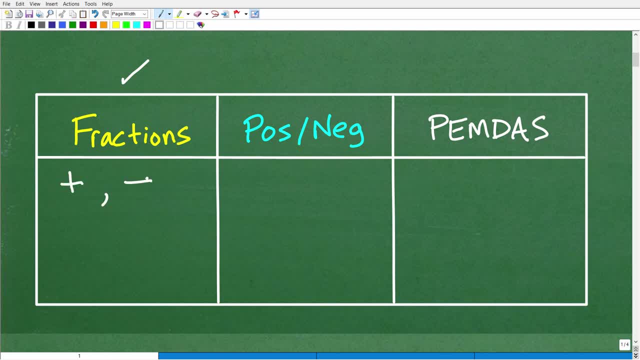 know how to add fractions. You're going to have to know how to subtract fractions. You're going to need to know how to multiply fractions and divide fractions. You're going to know how to to find the lcd. you're going to have to know about mixed number fractions- all that good stuff, just. 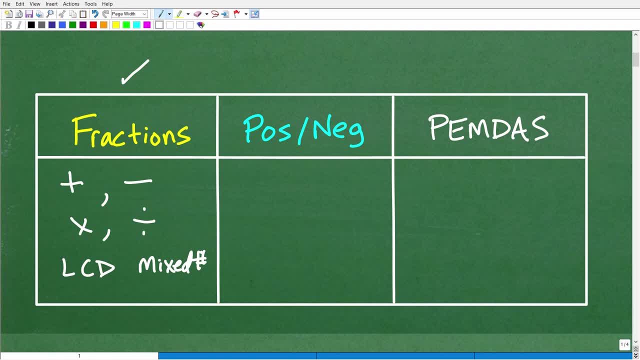 become like master fractions, the best of your ability. they're not going away. you're going to see a lot of them and you've been studying fractions. you know when you get the eighth grade level. you've been studying them year after year after year, just a little bit at a time. a. 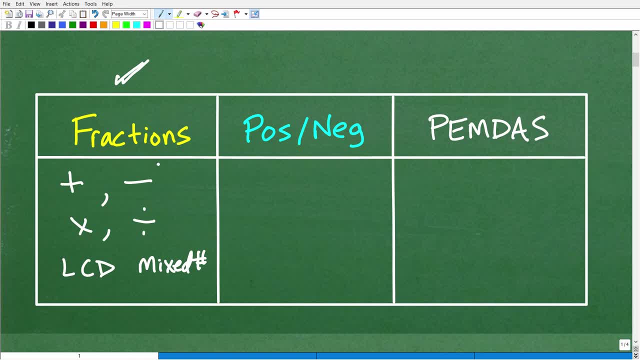 little bit at a time, but you really, at this point at the eighth grade level, you should be able to handle, uh, pretty much any fraction problem. another thing in here, too, is how to reduce fractions. so there's a lot to know in the area of fractions. now i'm going to give you a suggestion. 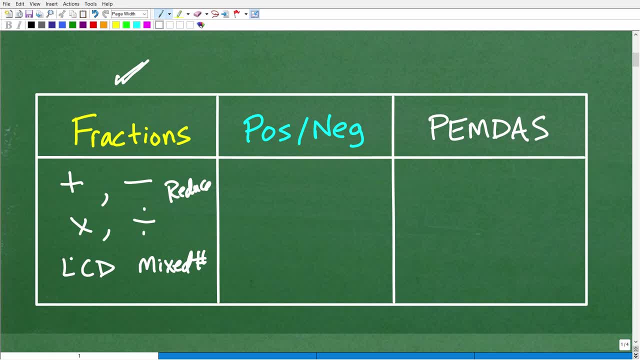 if you are reviewing, um, you know right now, if you're looking at doing some math review and i'll say, okay, fractions, how do i get, how do i learn fractions? well, a couple suggestions. one: i have tons of videos on fractions in my pre-algebra playlist on my youtube channel. 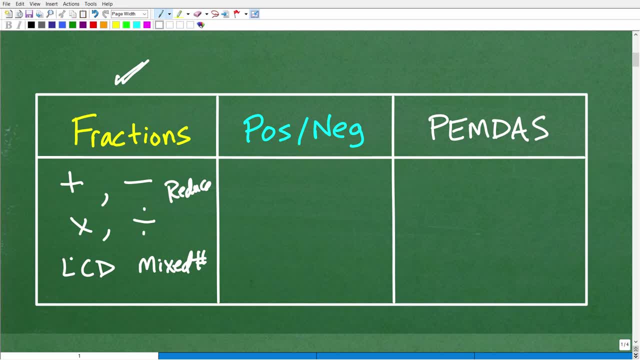 definitely want to check those out. actually, they have millions of views- some of my videos, so there's a lot of videos on there and i'll see you in the next video. bye of people looking for uh fraction help, but if you really, really want to learn this stuff, i'm going to. 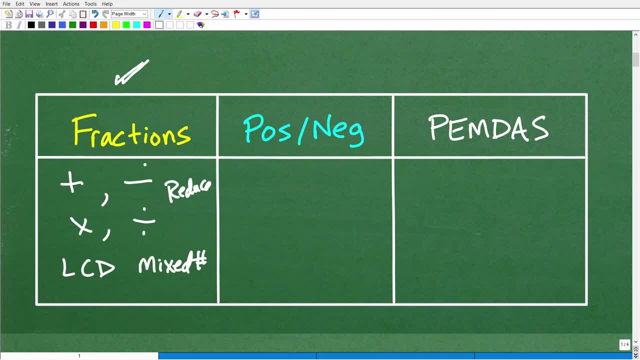 give you two courses in my math help program that i would recommend. the first i would recommend is my pre-algebra course, but i also have a math foundations course which goes into more basic math, like how to multiply numbers, divide numbers, just basic arithmetic. so that's called my math. 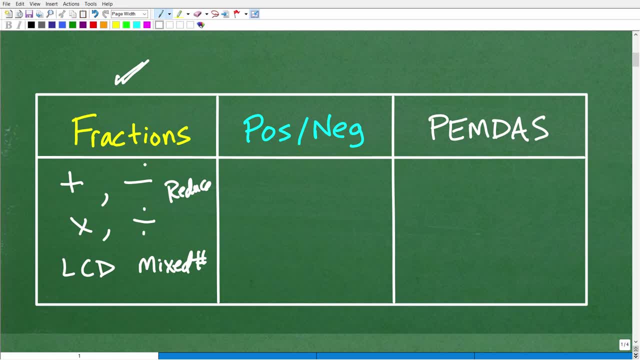 foundations course. you can find all that in the middle in high school math category in my math program. but uh, that course, or my pre-algebra course, would be excellent reviews for these topics that i'm talking about. okay, so fractions: if you can become an expert at fractions, you're going to be in super 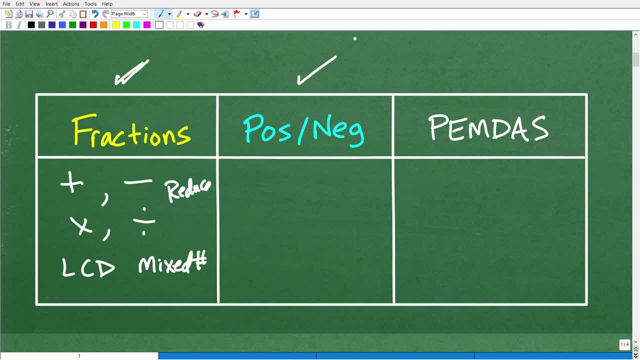 good shape, all right. the next thing is positive and negative numbers. a lot of students confuse this. okay, how do you multiply? let's say negative three times a positive two. or how do you divide negative 10 divided by negative five. this is actually easy, but it's also easy to mess up. 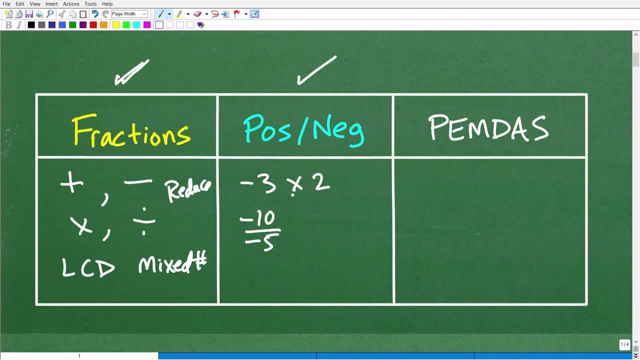 okay, you can't be guessing. you've got to be able to guess what's going on here, so i'm going to show you how to really master this stuff. so how to multiply, how to divide and how to add and subtract positive and negative numbers- very, very, very important, just like fractions. fractions are not going away in. 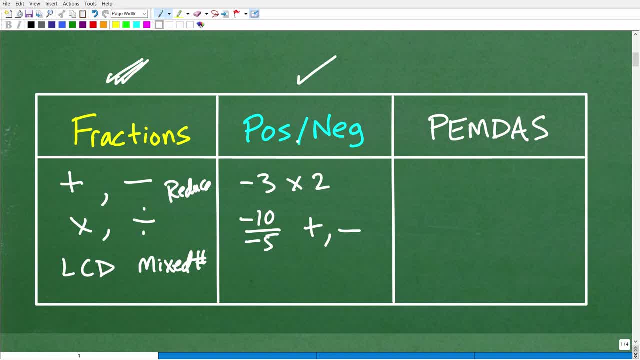 algebra. you're just going to see more of them and you're going to see a ton of positive negative numbers all the time, and you're also going to see positive negative fractions. you're going to be dealing with things like negative two-thirds plus a positive one-seventh. so you know it starts to. 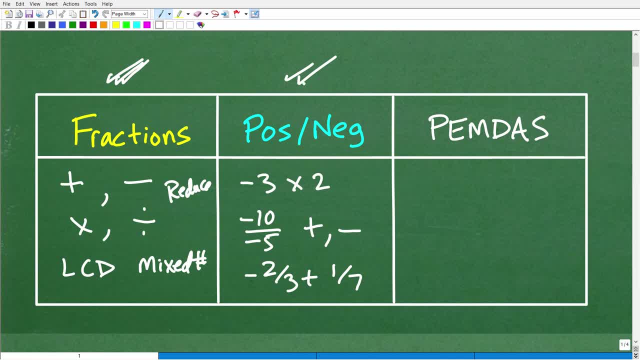 count on itself, right? so again, fractions and positive negative numbers- hugely important. you're going to see this constantly, all right, so what is this last one here? okay, so i kind of uh, have it written as pemdos. that should mean something to you. and this is the order of operations, okay so? 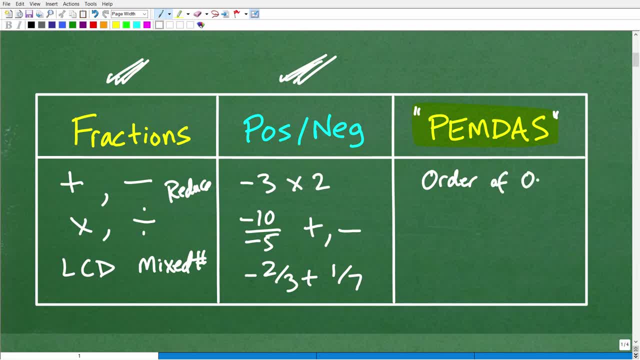 this is the order of operations. okay, so p stands for parentheses first. and, by the way, this little monic, a little a, that goes along, that's. most people were taught this little phrase or something like it. so that is, please excuse my dear aunt sally, okay, so that's one way to remember it. but 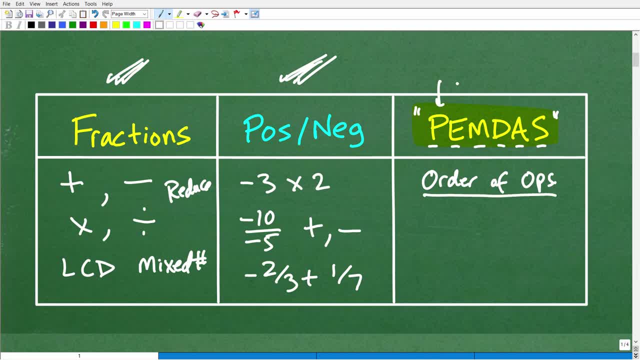 it's the order of operations. so the p stands for parentheses, the e stands for exponents or power, and then we have multiplication, division and addition and subtraction. i'm not going to try to teach you all of this and, uh, teach you these things in this video. i'm just telling you these. 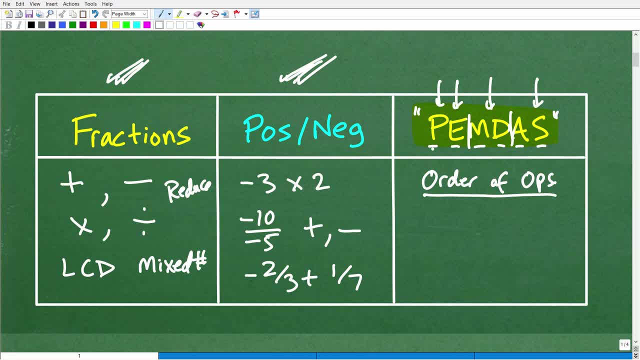 and a lot of students make um errors with this. they don't know this as well as they think they know it, okay. so again, i have videos on my youtube channel that go over this stuff and i thoroughly teach this stuff and those two courses that i met. but this is the order again of operations. 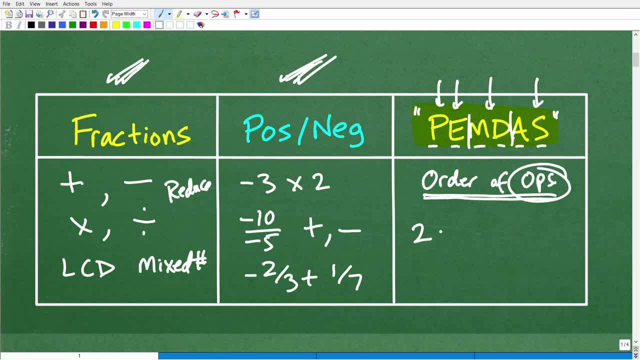 now, what are we talking about? mathematical operations. well, let's, let's take a look at a problem like this, okay, and i'm just making something up here, okay. so let's say, in this particular problem, i gotta do all. there's a lot of different mathematical operations. okay, a mathematical operation is addition, subtraction, multiplication, division and 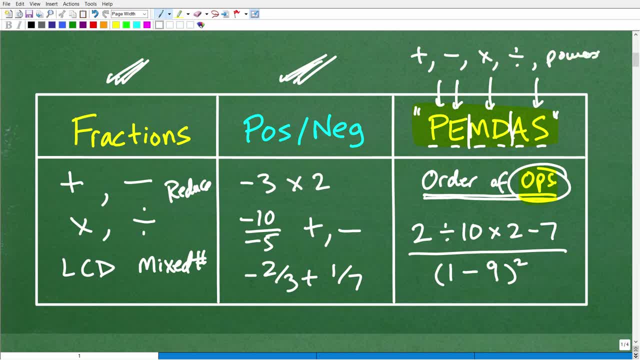 like powers. okay, it's things i can do with two numbers. i can, like you know, add them up or i can subtract them, etc. so that's what an operation is. so the order is: well, what order do we do first? because if we take different orders, if we divide or if we multiply, then uh, do that first. well, that's. 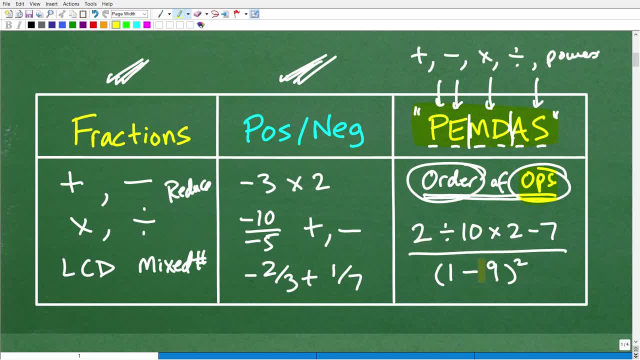 if i divide first, okay, you could just do these problems on your own. i can come up with all kinds of answers depending on what order i do these operations, and so this pemdos tells me- it's a checklist- do these, uh do a problem like this, with various operations in it in this specific order. 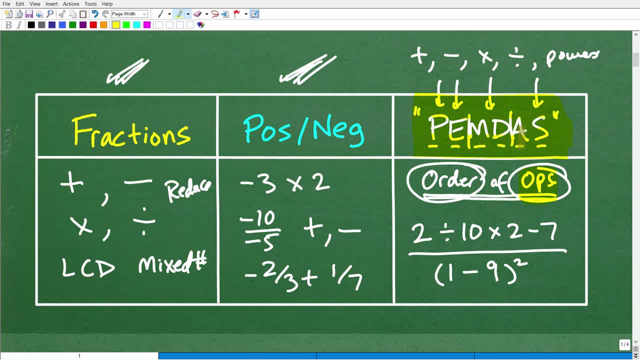 you got to really really understand this stuff, okay. so again here we have division, multiplication, subtraction, we got a fraction bar, we got another subtraction and we have a power. so what's the order we need to get out of here, okay? so what's the order that we do? the multiplication subtraction? 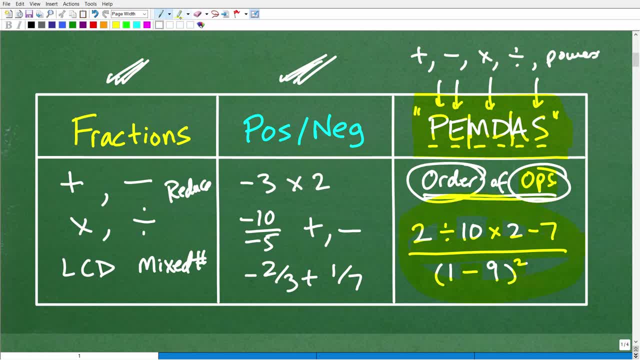 we have a fraction bar, we got another subtraction and we have a power, so what's the order we need to to do this in? well, that is PEMDAS. that's the order of operations. you got to know this, okay, so let's go ahead and wrap it up at this point. if you understand the order of operations, super good. 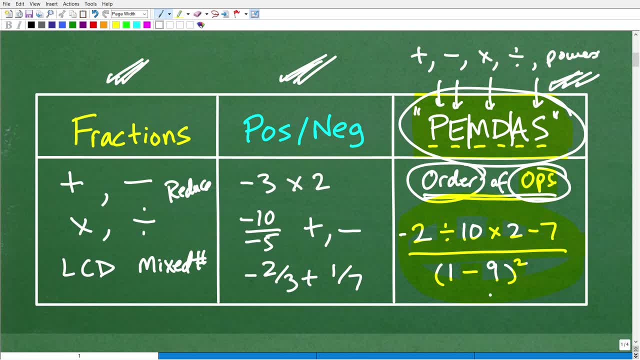 and, by the way, you can have negative numbers in here and you can have fractions as well, so it can get quite complicated. what from like a at an arithmetic level? we haven't even done anything with algebra and variables. okay, so you can see, you know, you got to give you know. eighth grade. 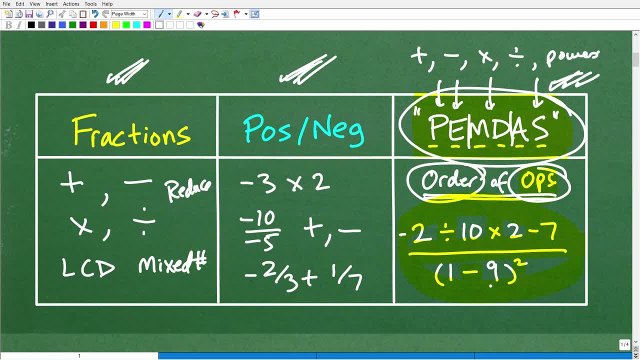 math, middle school math. it's due respect. you are doing a lot of you know. you know this requires a lot of focus, let's say, and knowledge and skills to be successful with arithmetic at this level. okay, so, order of operations: positive, negative numbers and fractions: you master all three of. 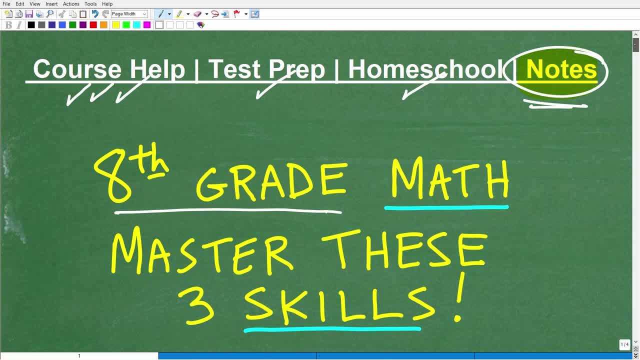 these things. here you're going to be sitting very, very nice for your next math class, which is likely going to be pre-algebra or maybe even an algebra one course. all right, so let's go ahead and finish this video up, if this was helpful, if you're like: oh okay, that sounds like a good uh set of suggestions. 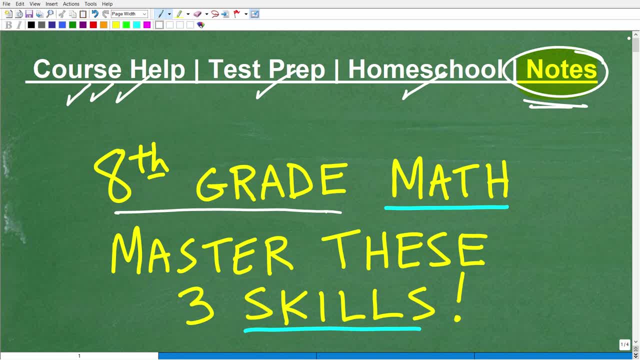 listen, i'm only, you know, been teaching this stuff for years and years and years and decades and decades. i'm teaching you from experience. i'm not telling you anything that uh isn't you know, uh backed up by tons and tons and tons of experience. okay, so follow me on this, all right, just like my.